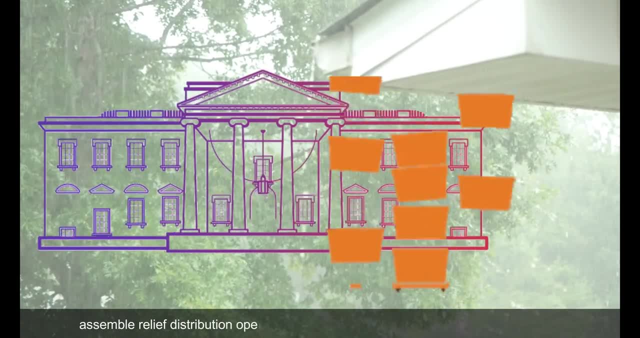 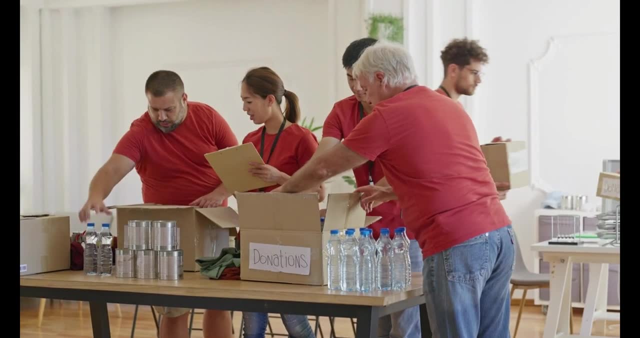 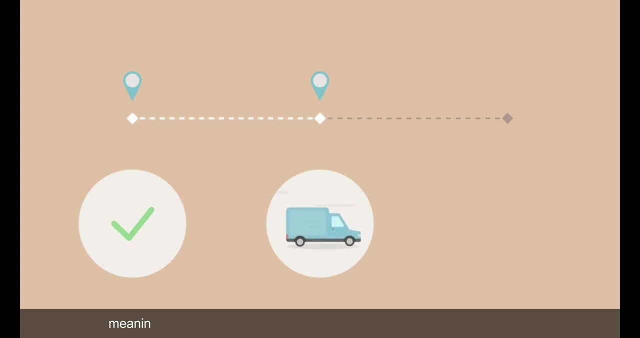 The government officials and volunteers assemble relief distribution operations with 13 barangays greatly affected by the typhoon. The question is: how can the government officials and volunteers distribute the reliefs in the most efficient way, meaning that they take the shortest paths to make the transportation costs less? 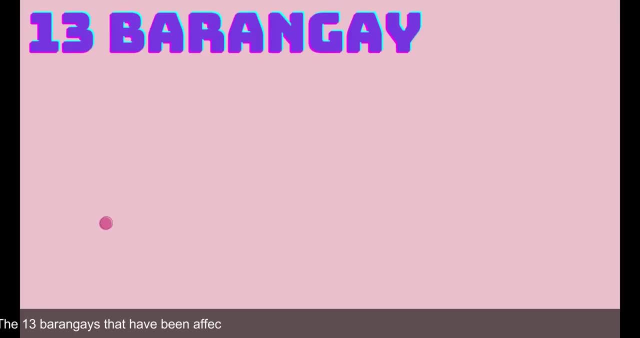 The 13 barangays that have been affected by the typhoon are: 1. Pitbitan, 2. San Nicolas, 3. Masantal, 4. Tabig, 5. Balubad, 6. San Francisco, 7.. 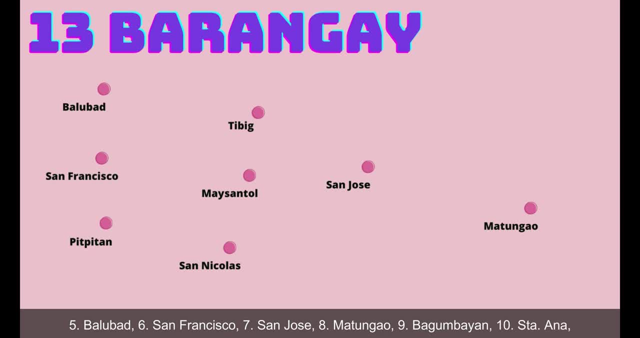 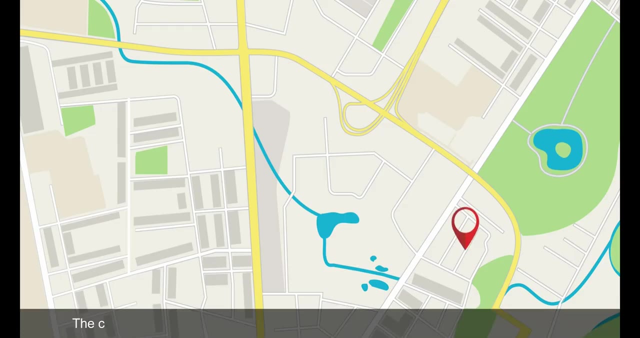 San Jose, 8. Machunau, 9. Bagmayan, 10. Santa Ana, 11. Santa Ines, 12. Bombong and 13. Perez- The concept that is used to find the shortest path for each of the edges to be traversed. 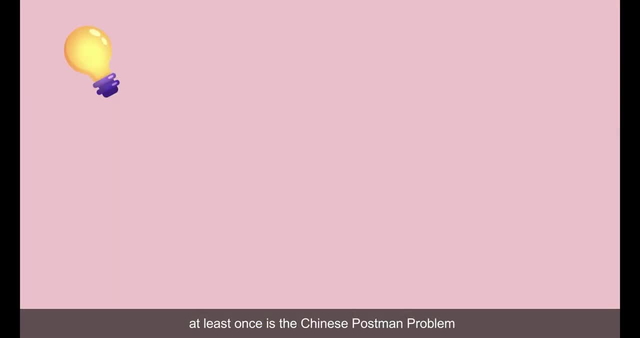 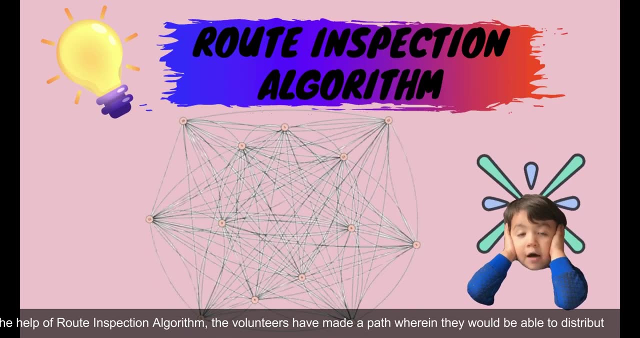 at least once, is the Chinese Postman Problem? With the help of route inspection algorithm, the volunteers have made a네요rsite of radio waves. You can see it at the top right corner of this video. You can see them have made a path wherein they would be able to distribute the reliefs. 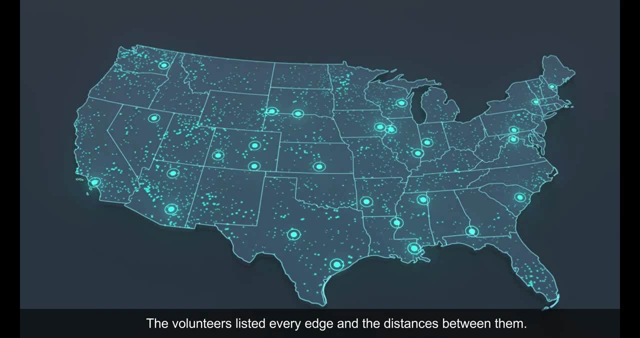 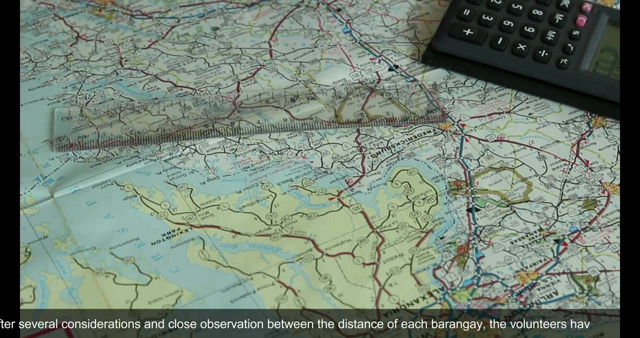 The volunteers listed every edge and the distances between them. The volunteers then proceeded to look at the shortest possible distance between every two vertices to see the shortest path that they can create After several considerations and close observation between the distance of each bar and guy. 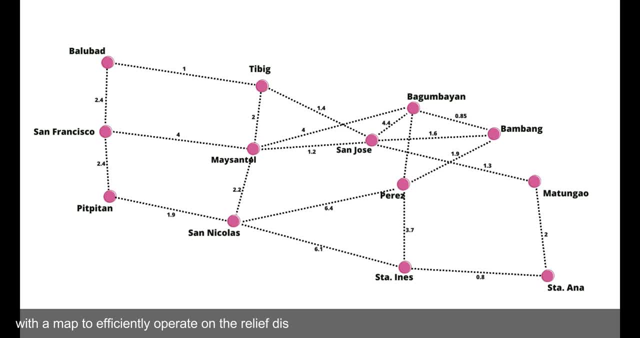 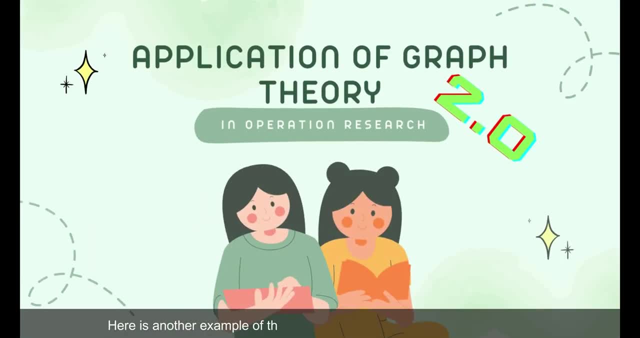 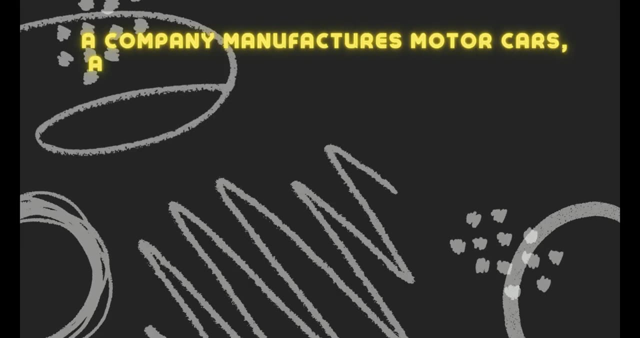 the volunteers have come up with a map to efficiently operate on the relief distributions. This is the map that the volunteers have created. Here is another example of the application of graph theory in operation research. A company manufactures motor cars and it has three factories- F1,, F2, and F3, whose 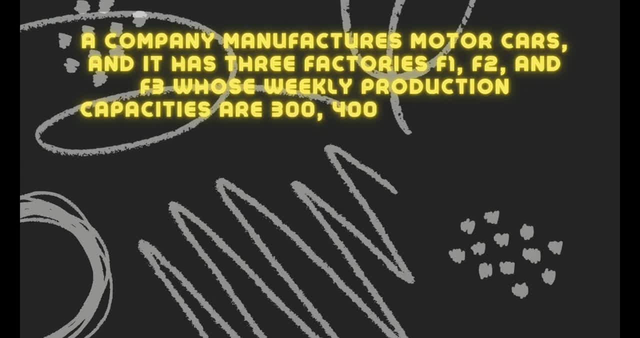 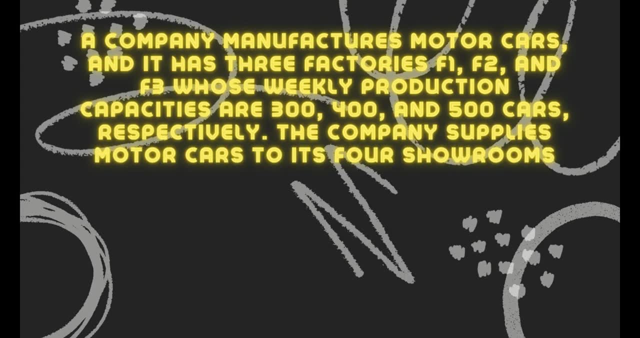 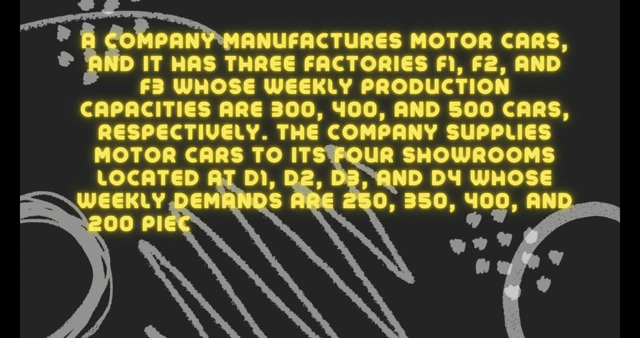 weekly production capacities are 300, 400, and 500 cars respectively. The company supplies motor cars to its four showrooms located at D1,, D2,, D3, and D4., Whose weekly demands are 250, 350, 400, and 200 pieces of cars respectively. 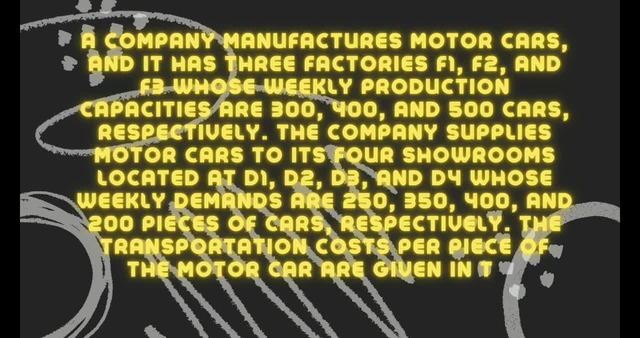 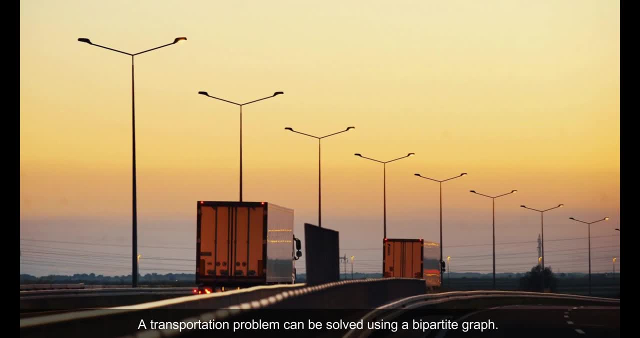 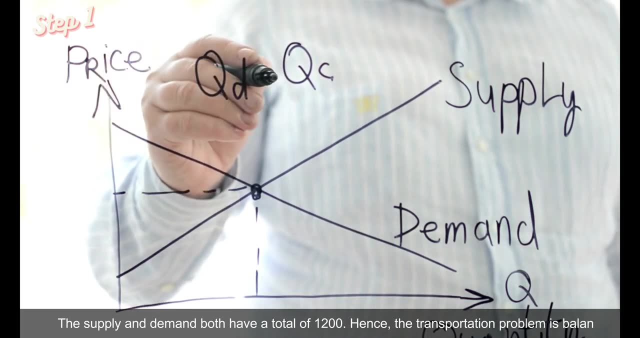 The transportation costs per piece of the motor car are given in the following: transportation: A transportation problem can be solved using a bipartite graph, Step 1. The supply and demand both have a total of 1,200.. Hence the transportation problem is balanced. 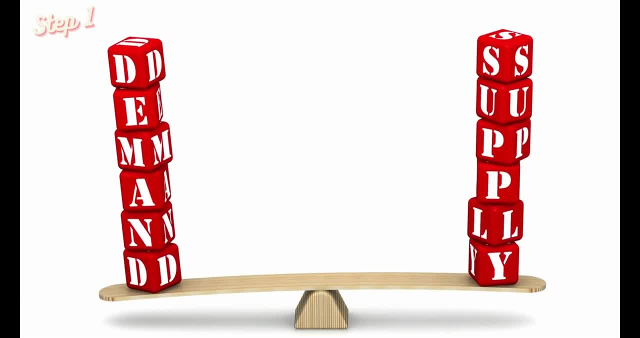 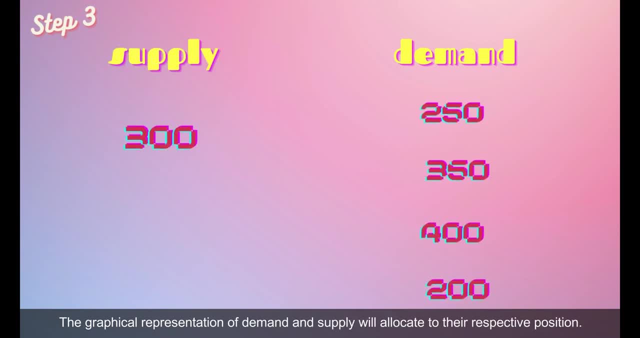 Since the problem is balanced, the transportation problem is balanced, Proceed to step 3.. Step 3. The graphical representation of demand and supply will allocate to their respective position. The demand will be on the right side and the supply on the left side. 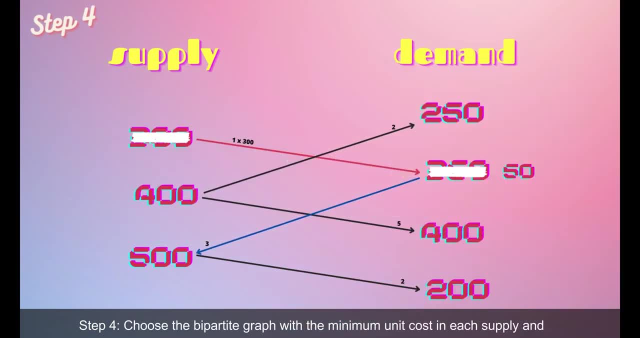 Step 4. Choose the bipartite graph of the minimum unit cost in each supply and demand: Step 5. Determine the edge with minimum unit cost t i j and allocate the minimum unit cost hedge- Step 6. The allocation begins from the edge that has the minimum cost and decreases the minimum. 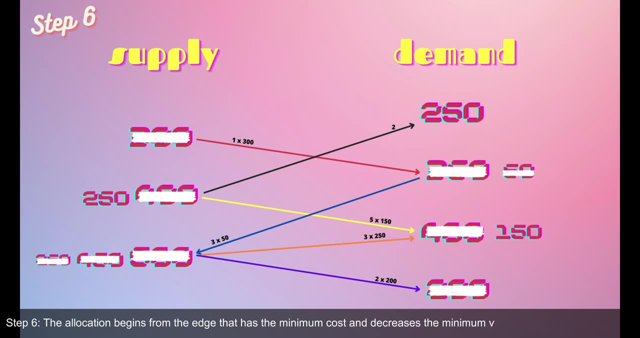 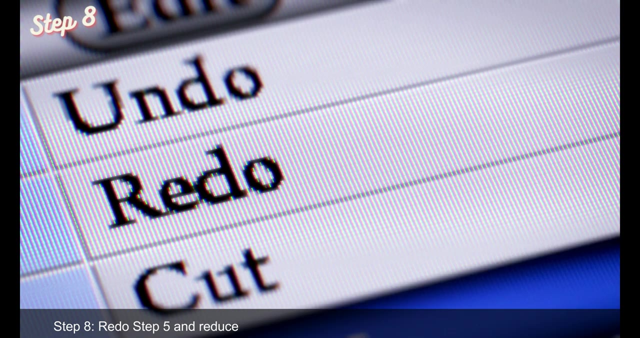 value of the vertices of supply and demand, along with the satisfaction of the condition of the bipartite graph- Step 7.. If the conditions of the graph have been satisfied, proceed to the next step, Step 8.. Reduce step 5 and reduce the minimum value from the vertices of supply and demand along. 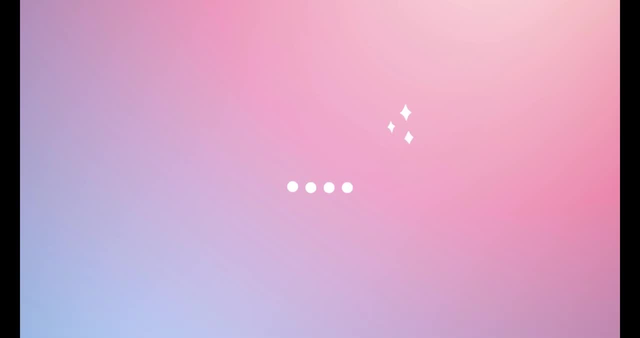 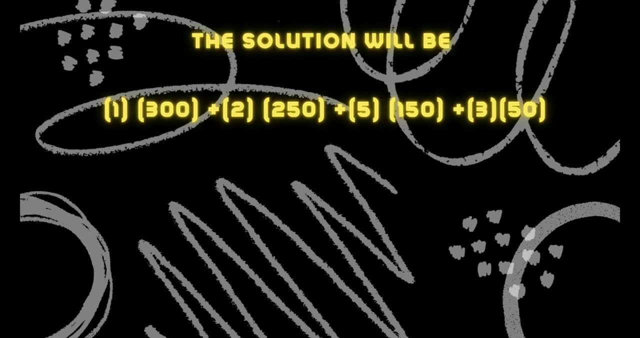 with the satisfaction of the condition of the bipartite graph, The solution will be: 1 times 300 plus 2 times 250 plus 5 times 150 plus 3 times 50 plus 3 times 2500 plus 20 times 200 equals 2850.. 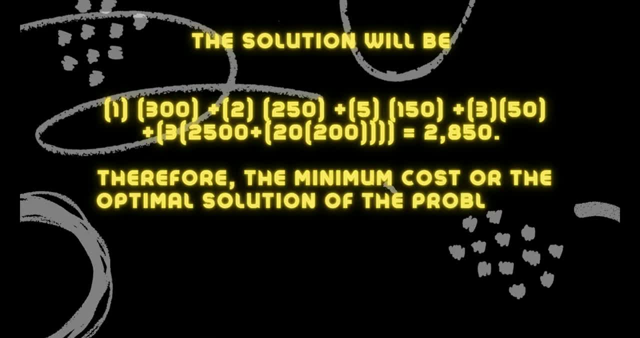 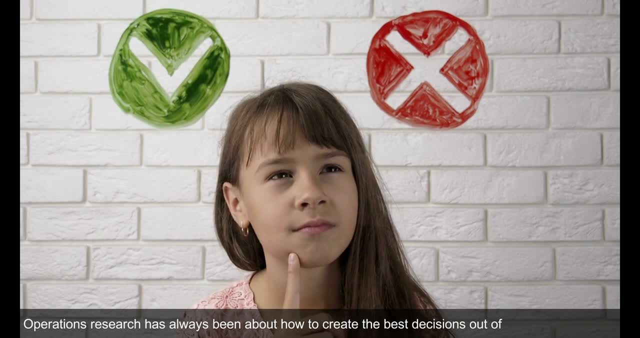 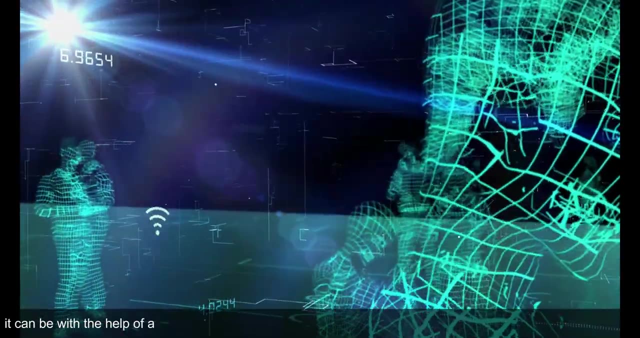 Therefore, the minimum cost for the optimal solution of the problem is 2850.. Operations research has always been about how to create the best decisions out of the limited options. It has come to light that graph theory could be a help in several ways. it can be with the help of a problem like the Chinese postman problem, or it could be of a simple bipartite graph. 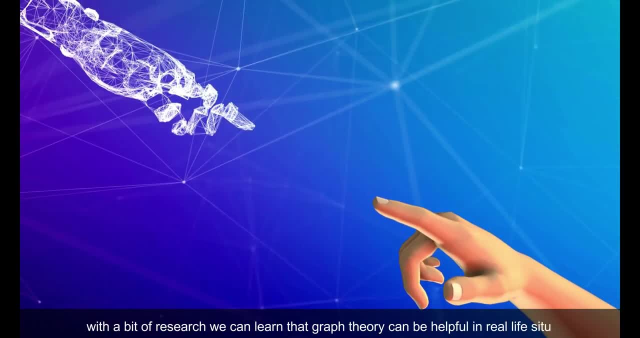 With a bit of research, we can learn that graph theory can be helpful in real life situations.